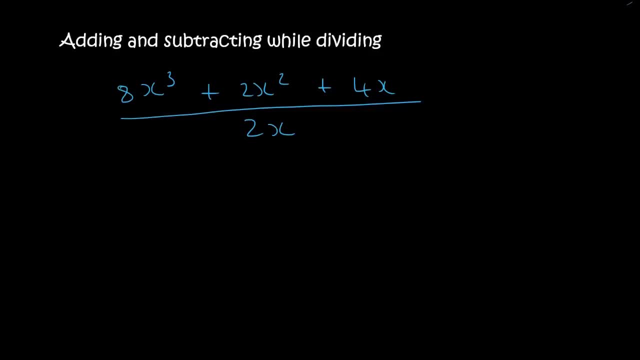 So students typically struggle with these kind of questions. Let me quickly show you. in the previous lessons we were looking at questions like this, where we had a multiplier in between, and so the 8 and the 2, did they have any exponents? No, they didn't. So what did we do? 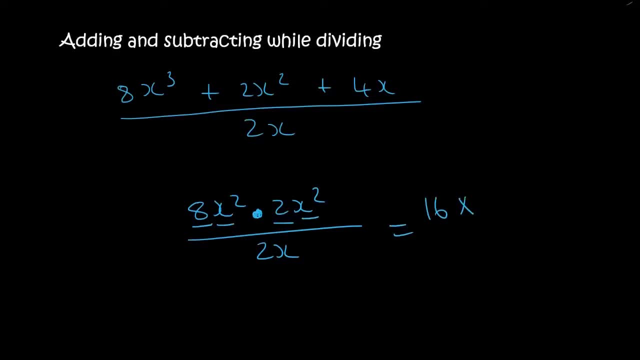 We multiplied Then the x and the x. you simply add their exponents, and so you get x to the 4, and then at the bottom we had 2x. Now 16 and 2, there's no exponents there, so you just divide. 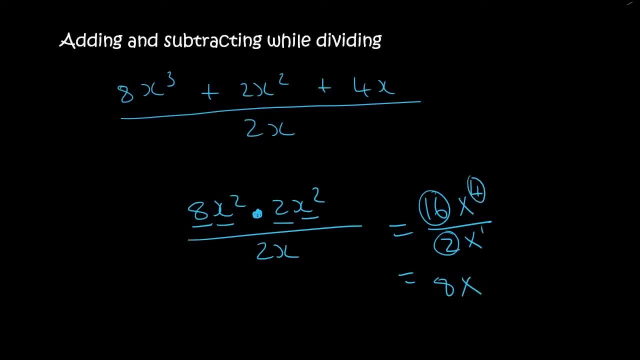 and that's 8.. Then with the x's, because they have the same base, you minus their exponents and you end up with 8x3.. But now carefully look at this and then look at this one. There is now a plus or it sometimes can be a minus in between. So we need a different approach. 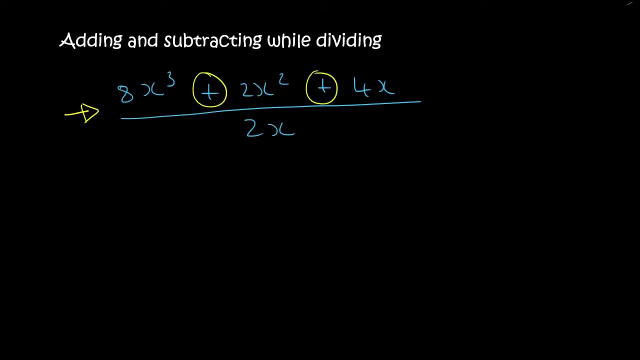 So maths is all about practice, and as you practice you'll start to see the different types. So what you do with these ones is you sort of take that part, then you take that part, and then you take that part. Let me show you that again, So you will take. 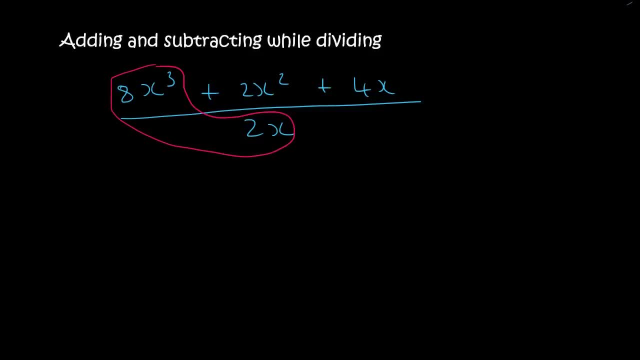 that part first We'll separate that so that'll become 8x3 over 2x. Then you take the next part, which is plus 2x squared over 2x, and then the last part is plus 4x over 2x. 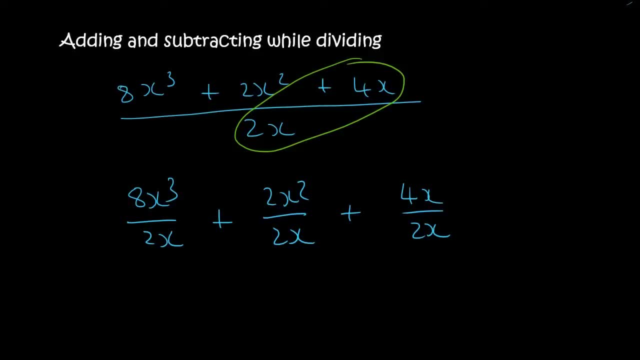 That's the difficult part. Now it's easy because in the previous lesson we looked at how to do ones like this: 8 divided by 2, well, the 8 and the 2 don't have any exponents, and so you can just say: 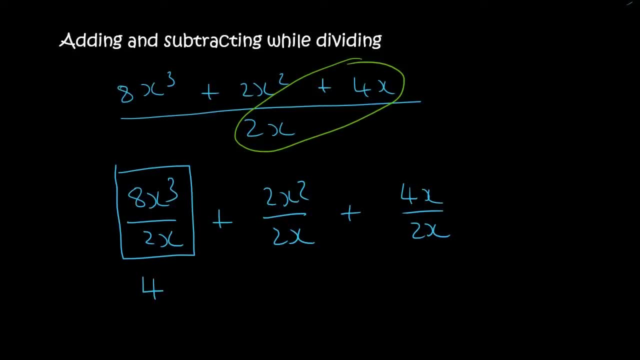 8 divided by 2, which is 4.. x3 over x? well, you just minus the exponents and so that just becomes x2.. 2 divided by 2 just cancels out completely, and then x2 divided by x1 just becomes x1. 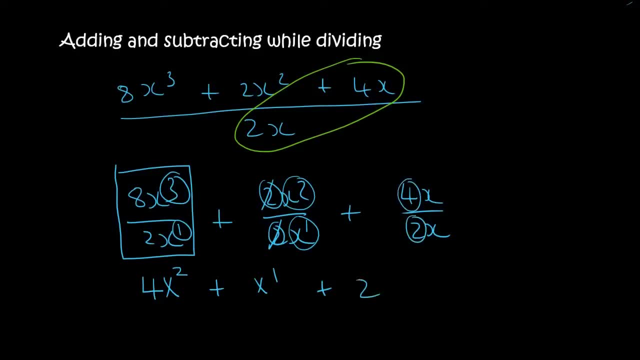 And then here we have 4 divided by 2,, which is 2, and then the x's cancel. If you want to be technical, this exponent here is a 1, and this exponent is a 1,, and so you should minus them, and so that will. 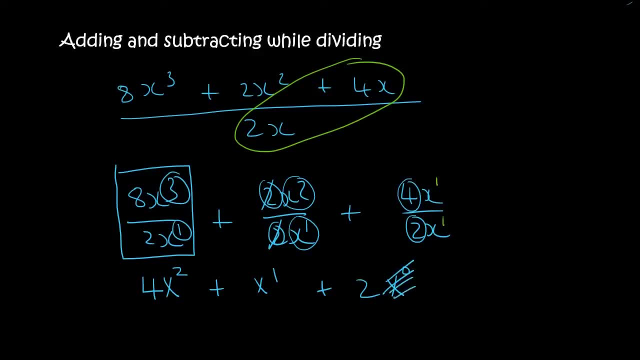 give you x to the 0, but anything to the power of 0 is 1.. And so the final answer is 4x squared plus x plus 2.. But, Kevin, shouldn't we put these together now? But guys, remember when we looked. 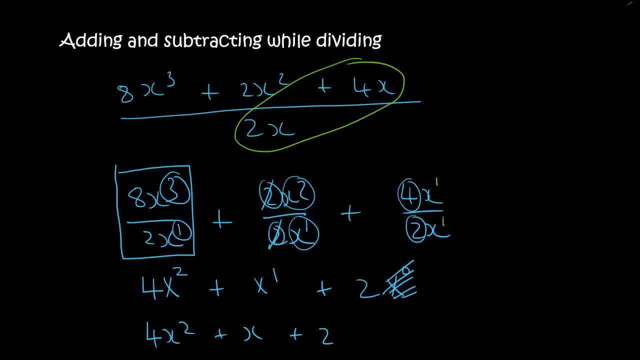 at the very first lesson of this chapter, we looked at how to add like terms, and so when you're adding like terms, we can only put them together if they are the same. Remember, in the very first lesson we looked at stuff like x plus x plus x squared, The x and the x are the. 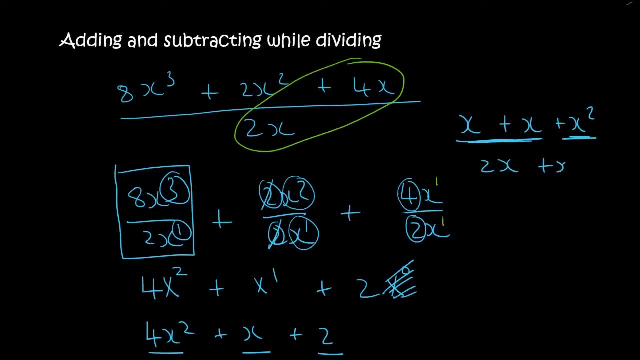 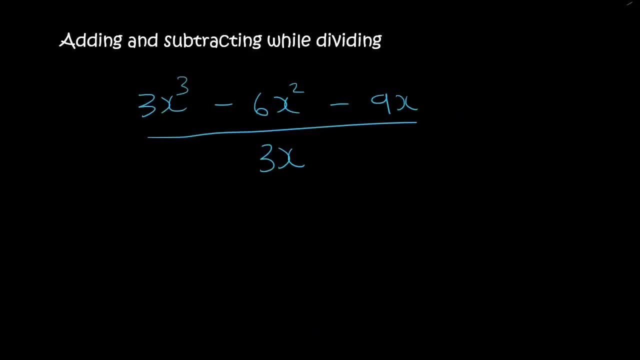 same, and so we said 2x, but then we couldn't add this part, And so this is the answer. So now we're just going to practice a lot of these. So here we go. So we've got minuses in between, So 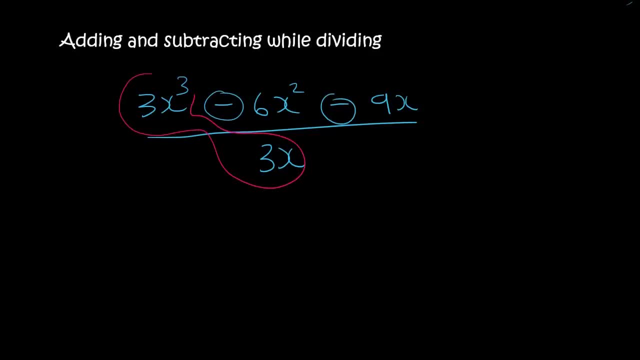 what we do is we isolate, So we take this one, and so that will be 3x3 over 3x. You then take over there, which will be minus 6x squared over 3x, and then you take minus 9x over 3x. 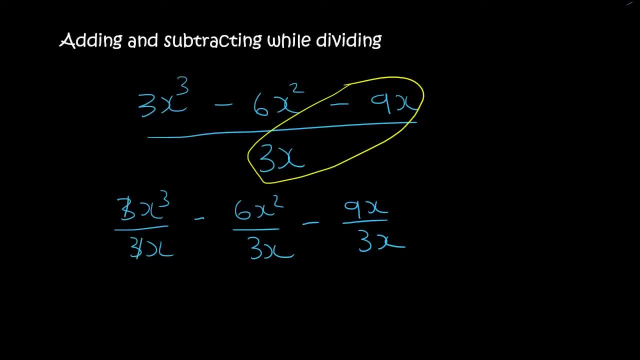 Now it's easy, because 3 divided by 3 is just 1, so you can say 1.. Then, if these are the same, then you minus the exponents, so you get x to the power of 2.. Then 6 divided by: 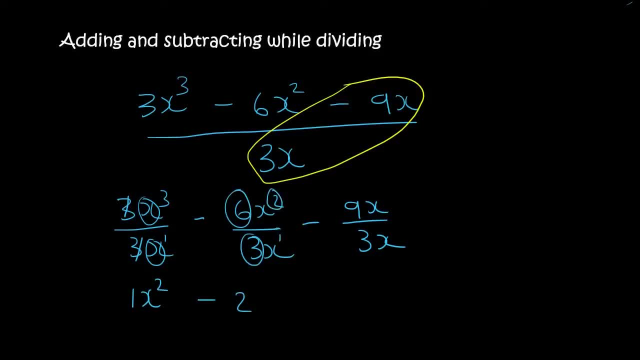 3 is 2, and then 2 minus 1 is 1, so it just becomes x1. And then 9 divided by 3 is 2, is 3.. x1 over x1 just becomes x0, but anything to the power of 0 is 1.. And so the final answer. 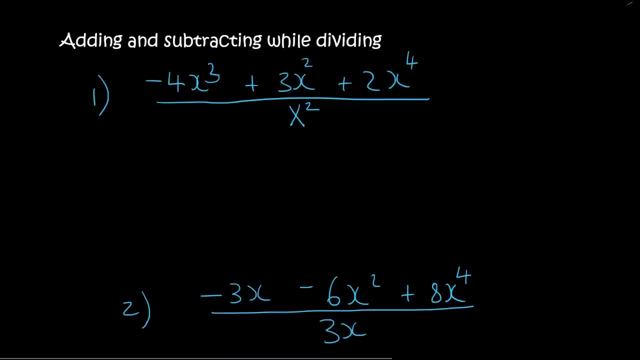 is x squared minus 2x minus 3.. So maybe you want to pause the video and try these two. So when we've got pluses and minuses in between, like that, we want to isolate. So we will say minus 4x3 over x squared. That was this part over this part. Then we say plus 3x squared. 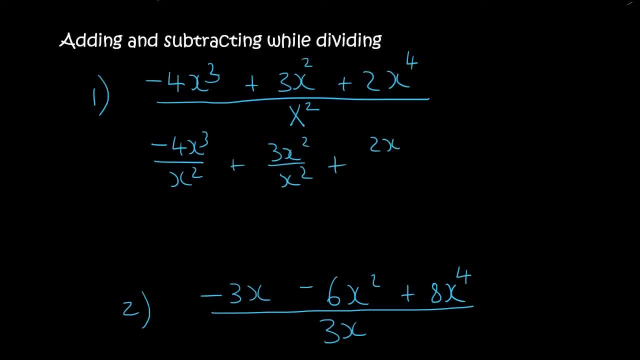 over x squared. And then the last part: 2x4 over x squared. That's the difficult part. This is the easy part. So 4 minus 4, there's nothing. there's no other number at the bottom, so that: 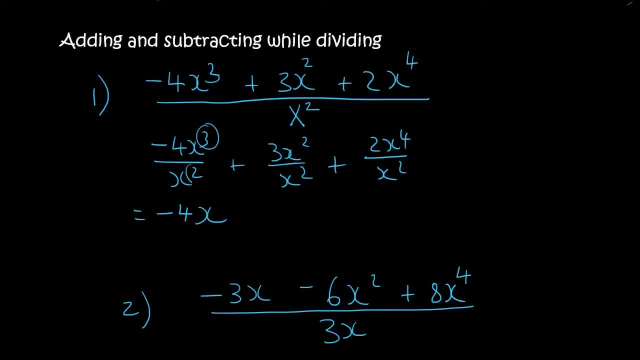 just stays minus 4.. For the x's you say 3 minus 2,, which is 1, plus this, just stays 3.. Now x2 and x2 becomes x0,, which is just 1, so you can ignore that part, And then this part just becomes. 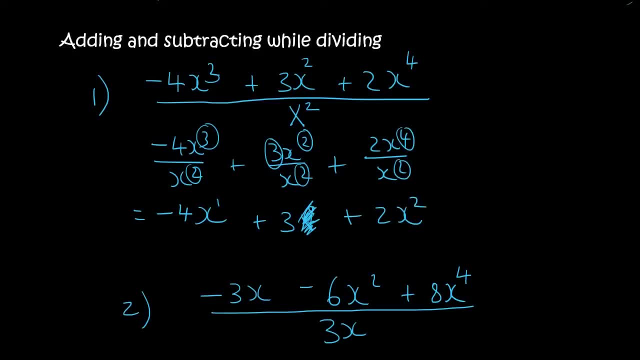 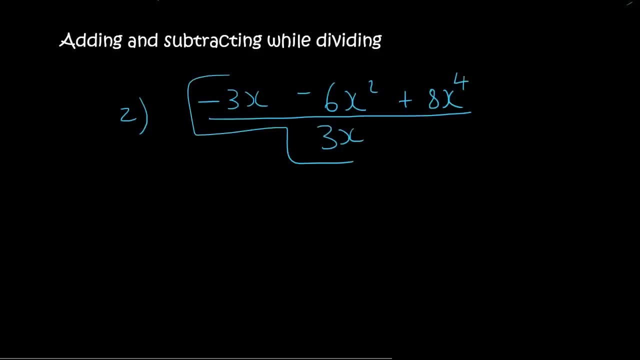 2x, and then 4 minus 2 is 2.. And so the final answer is minus 4x plus 3 plus 2x squared Number 2.. So what we do is we first isolate that part, So we write it as minus 3x over 3x. 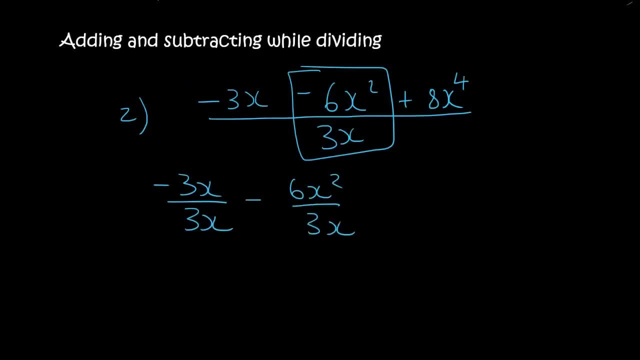 Then it's minus 6x squared over 3x, And then it's plus 8x4 over 3x. So here we go. If you want, you can type this in on your calculator: Minus 3 divided by 3 will just give you minus 1,. 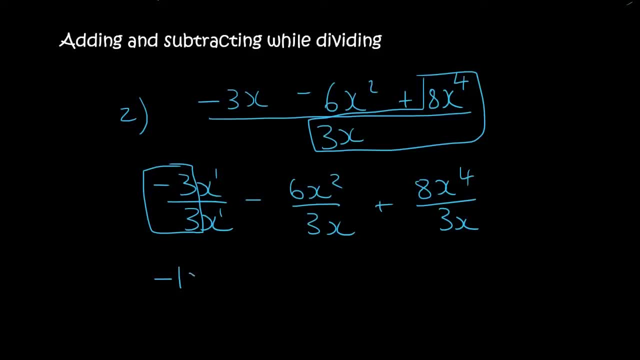 x1 over x1.. If you minus the exponents you get x0. Now x0 is just 1, so you can ignore that 6 divided by 3 is 2.. Then 2 minus 1 is 1.. 8 cannot divide by 3, so we just leave it. 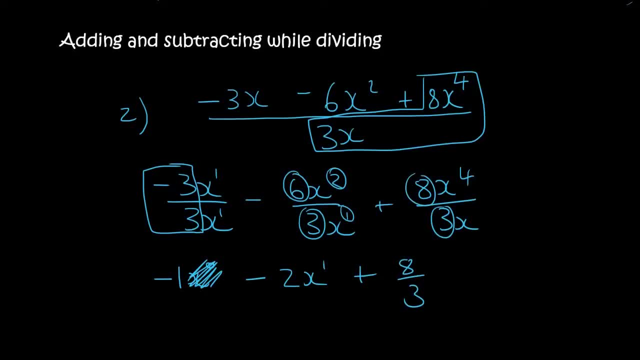 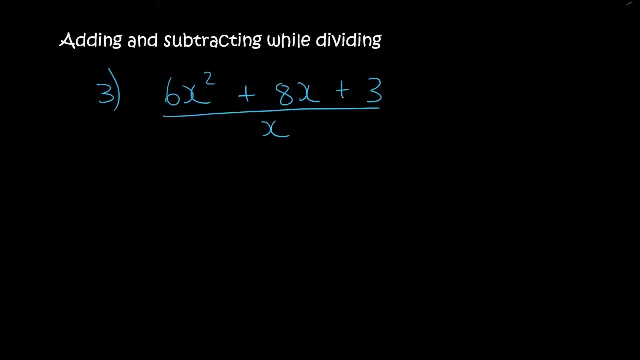 as 8 over 3.. And then x4 over x1 becomes 4 minus 1, and that's just x3, number 3. So we isolate it. So it's 6x squared over x plus 8x over x, plus 3 over x. So 6 is just going to. 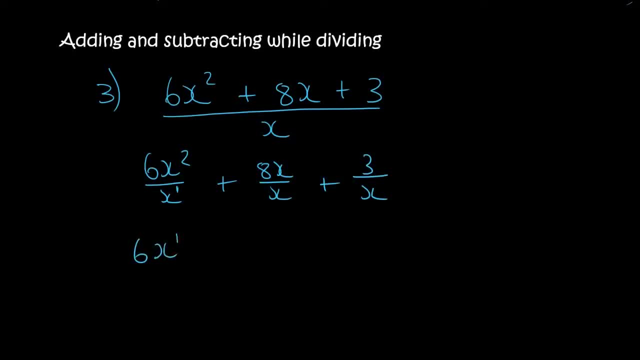 stay 6.. This is a 2 minus 1, which just becomes x to the 1.. 8 will just stay 8.. And then the x1 and x1 becomes x0 if you minus them. But then that just cancels, because anything to the power. 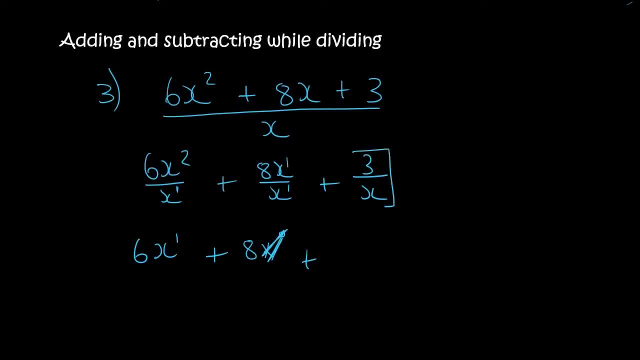 of 0 is 1.. And then when you get a situation like this where you've got an x and you've got an x at the bottom and nothing at the top, then leave it just like that. That is the answer. 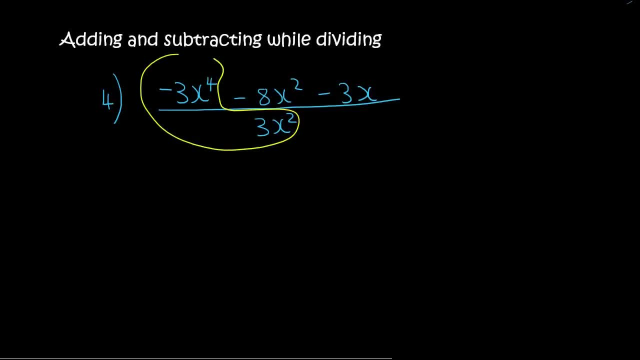 So we isolate everything, So we take that part first, So minus 3x4 over 3x squared. Then we take the middle part And then we take that part over there. That's going to be minus 3x over 3x squared. Okay, so now minus 3 divided by 3 is just minus 1.. 4 minus 2,. 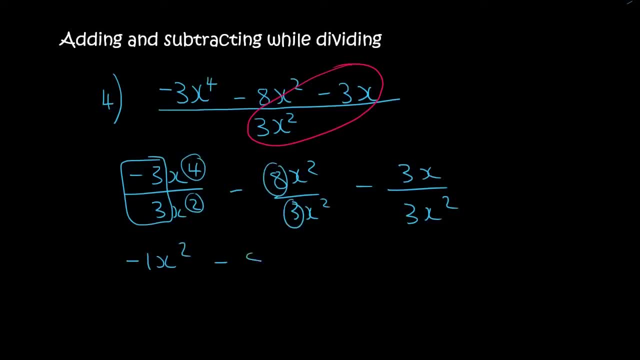 becomes x2.. 8 over 3 doesn't work, So you just leave it as 8 over 3.. 2 minus 2 is 0.. So that's x0.. But remember, that's just a 1.. So we ignore that. So it's just 8 over 3.. And then this one's: 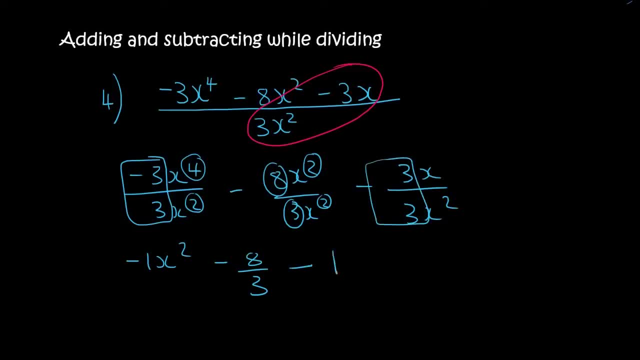 quite interesting. So it's minus 3 divided by 3, which is just 1.. Now we have an x1 at the top and an x2 at the bottom, And you should always say top minus bottom. So that's going to give you 1. 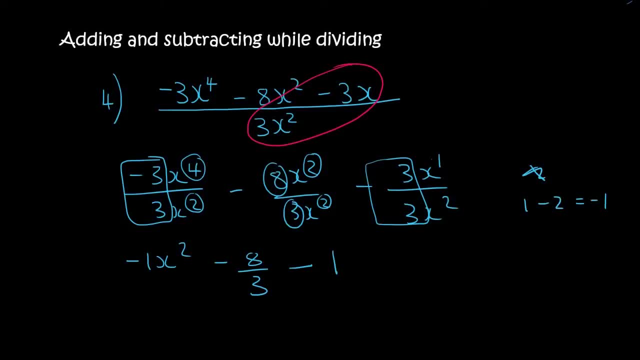 minus 2, which is minus 1.. So we haven't looked at this in this chapter yet, So that's going to be going to be x to the minus 1.. Now, a rule in maths is that you're not allowed to write your answers. 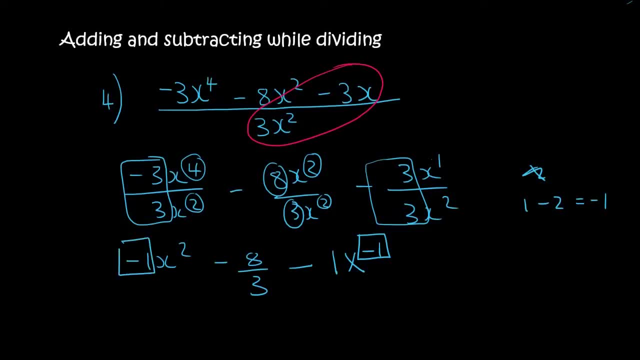 with a negative exponent. This is okay. that's not an exponent, and so what we're going to do is we're going to have to rewrite that number in a different way. So what we're going to have to do is to make this a positive again. you're going to have to take it to the bottom, So this 1 can stay where it is. 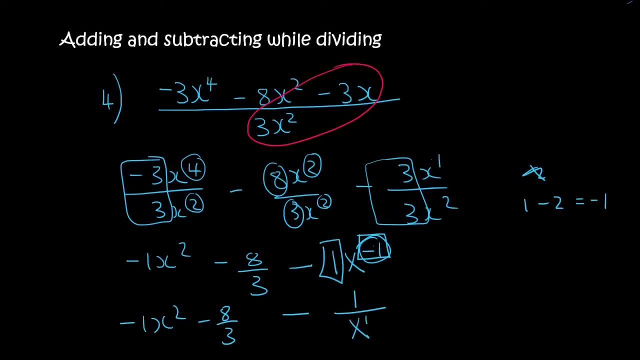 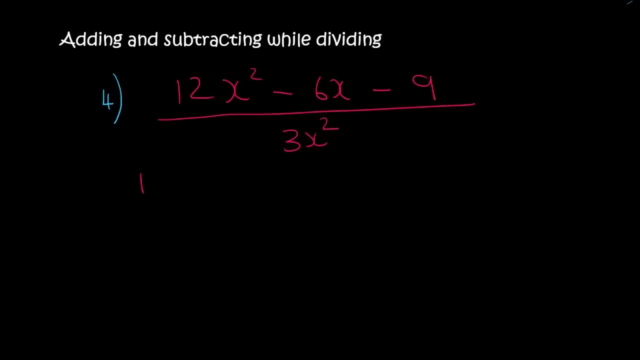 then at the bottom you'll just have x, but now it will be positive 1, and that's your answer. Let's practice a few more of those, All right? so here we go. so we isolate it first, so it's 12 x. oh no, this is now number 5, so it's going to be 12 x squared over 3 x squared minus 6 x over 3 x. 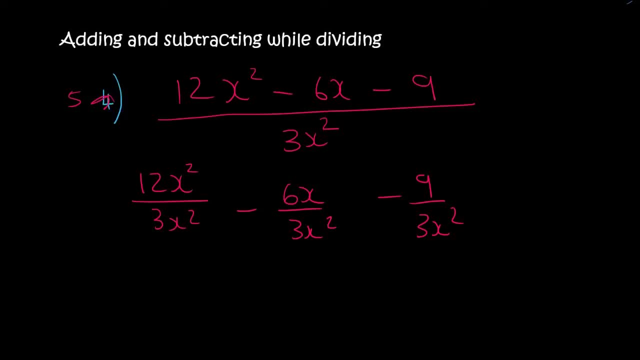 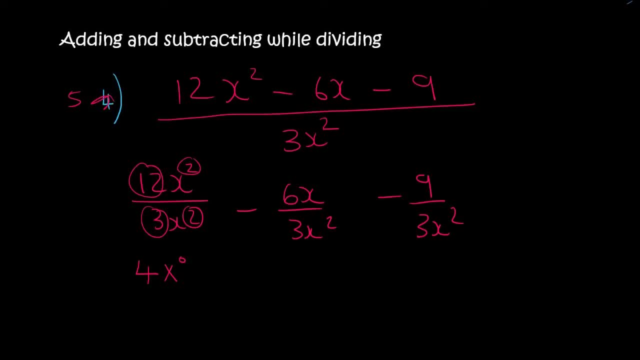 2 minus 2 is 0, and so that part actually just falls away. then we've got 6 divided by 3, which is 2. now we have 1 minus 2, which is minus 1, and then, when you already have something like this one, 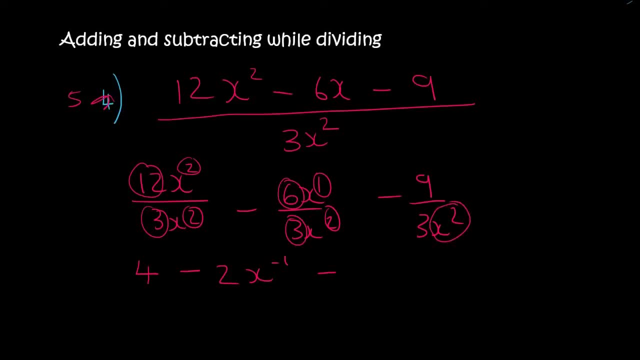 where the x2 is already at the bottom and it's positive and there's no x at the top, then just leave it just like that. however, 9 divided by 3 is 3, and then at the bottom, you've still got x squared. now we see, here we've got a negative exponent. so what we do is we 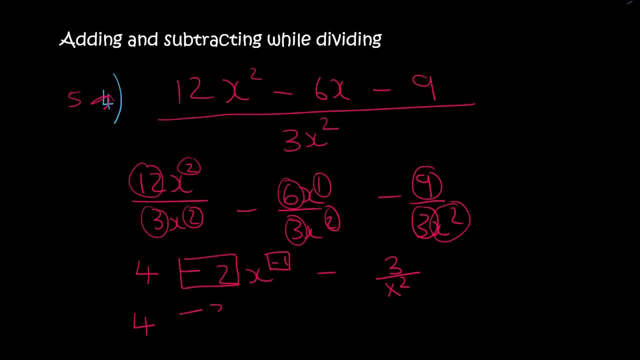 so this minus 2 is fine where it is, but this x minus 1 will have to go to the bottom, like that, you see. so we don't take, we don't take this whole part to the bottom, because the minus 2 is fine. it's the x that has the negative exponent, so that needs to go to the bottom.